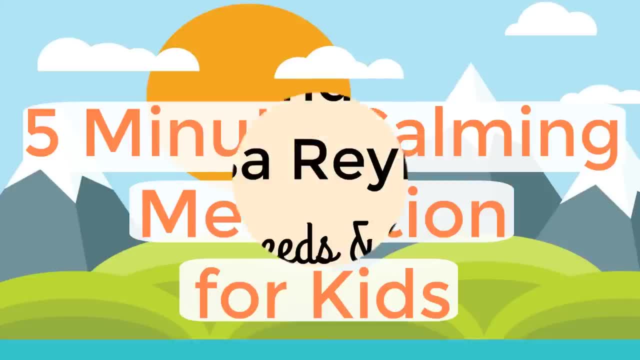 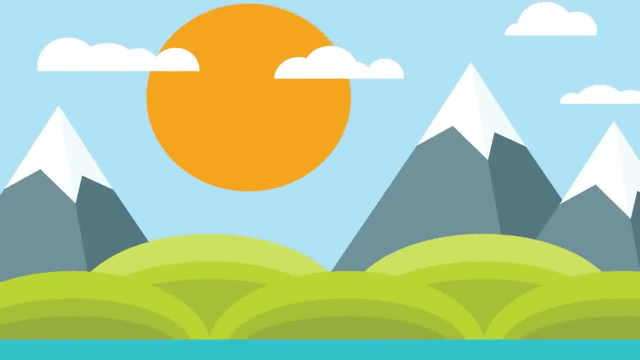 Hello, this is Alyssa Reynolds from flaxseedsandfairytalescom. Today I'm going to share a short guided meditation for kids. This meditation is just five minutes long and has calming music. Get ready to relax and join me on this lovely adventure. 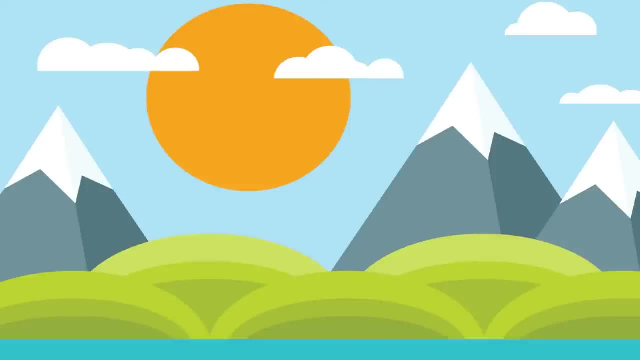 First, start by finding a comfortable position. You can sit up or lie down, whatever works best for you today. Now let's take two deep breaths together. Take a big breath in through your nose And out through your mouth. good job, let's try that one more time. a big breath in. 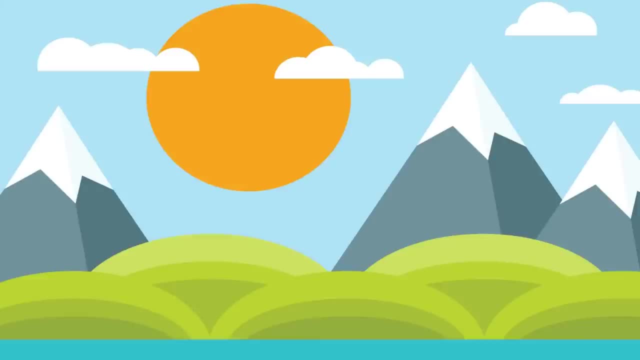 through your nose and out through your mouth. it feels so nice to just breathe. you can feel your whole body start to calm and feel really good. now imagine yourself in a place that you like very much. you can feel your whole body start to calm and feel really good. 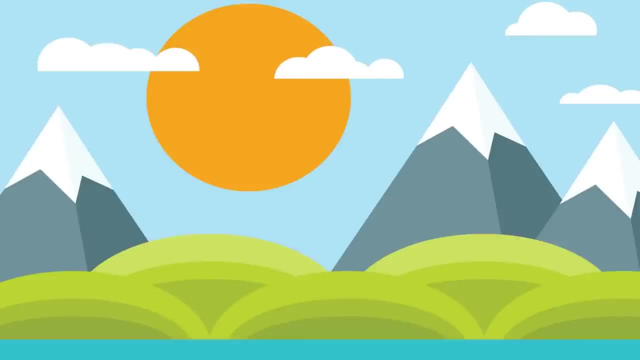 this could be the beach, or maybe the park, or even your own bedroom. just think of a place that makes you feel calm and happy. imagine yourself there right now and let's take two more deep breaths together. take a big breath in through your nose and out through your mouth.